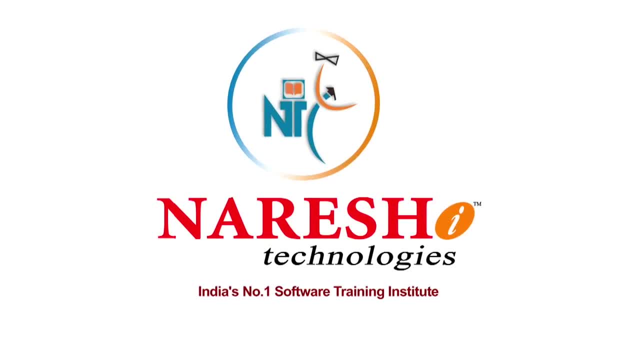 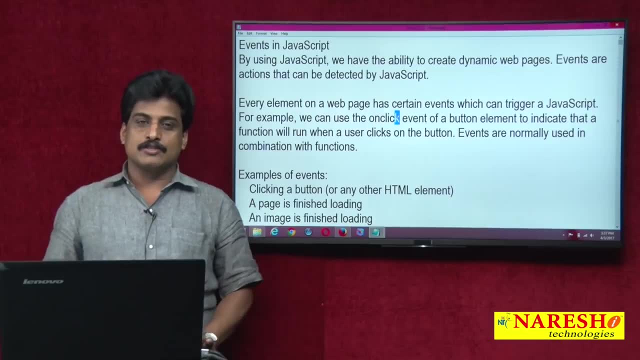 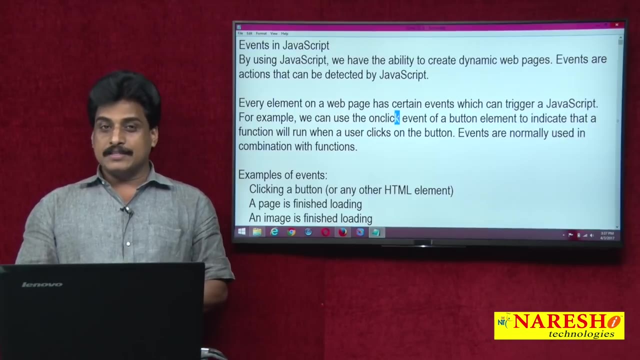 Hi guys, welcome to Narayansha Technologies. This is Subbaraju. In this video session you can view JavaScript events. What is an event? What are the events we can perform on the objects? Total how many number of events existed in JavaScript Like this? many other things we 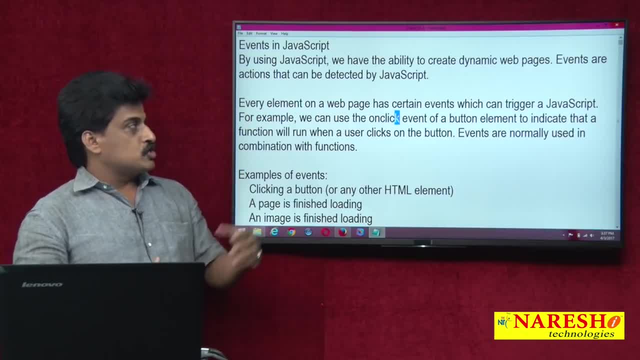 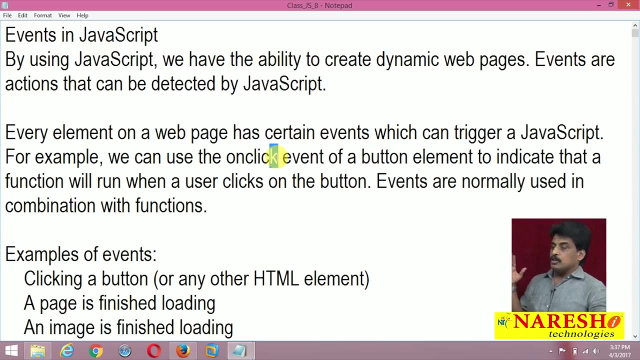 can discuss in this video session. By using JavaScript, we have the ability to create dynamic webpages, Definitely. that is a reason DHTML we are calling Dynamic Hypertext Markup Language, with JavaScript Events or actions that can be performed or that can be detected. 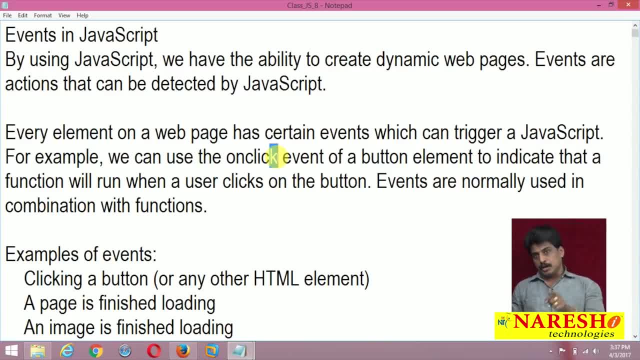 by JavaScript, performed on objects detected by JavaScript. And finally, I wrote here very clear: Events are normally used with the combination of functions. I am not saying without function also okay, But generally we are using with the combination of functions. A big list of 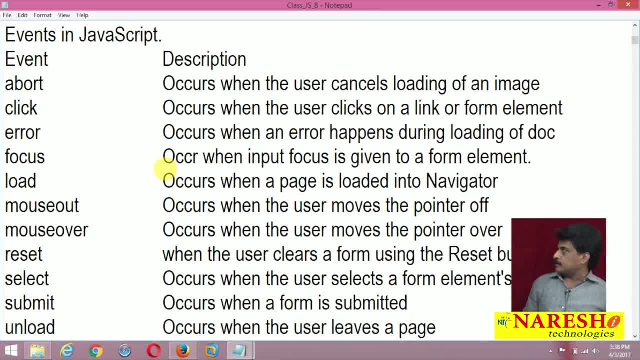 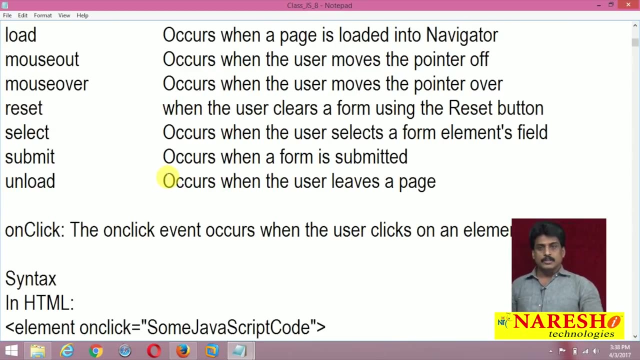 events existed in JavaScript, At least a few events you can try to observe here: Abort click error, focus, load, unload, mouse out, mouse over, reset on blur on focus. like this number of events existed, A few events before we are going to discuss So common event Almost. 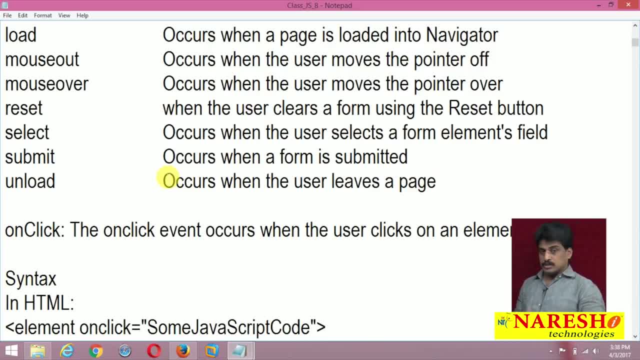 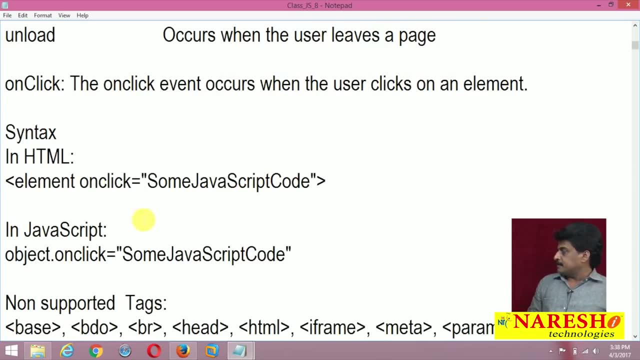 all maximum in video sessions are used mainly in JavaScript related video sessions. on click event: This event always fires when user click on the object: Single click. Now syntax, element level, JavaScript level. First I will show you element level Some JavaScript code When. 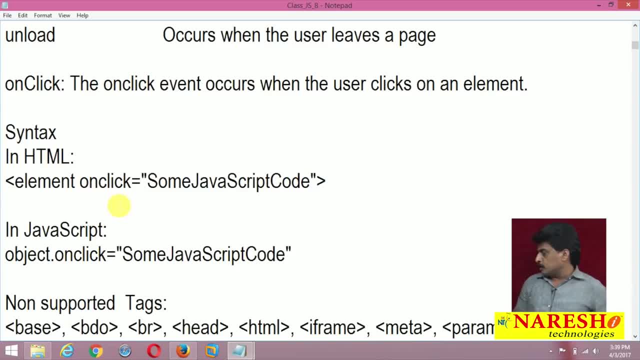 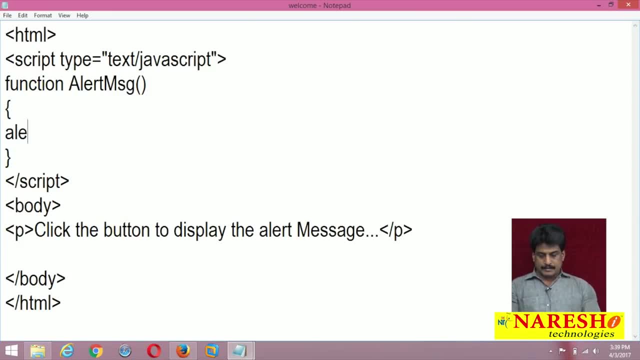 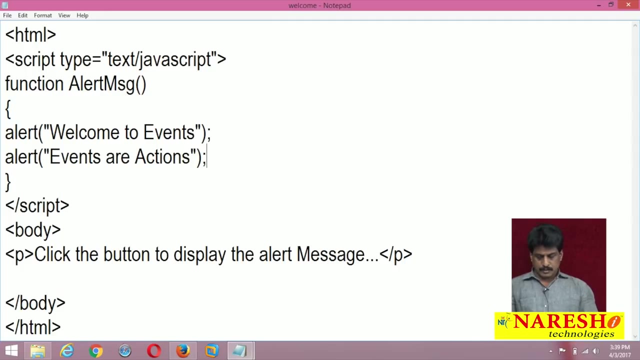 object basis: started. object level: click Now. if you are coming down support, non-support available. first we will go to direct example alert function. function name alert. Welcome to events. Alert events or actions. Come down to button. onclick is equal to non- enabling examples. All right, If I want to, all very. 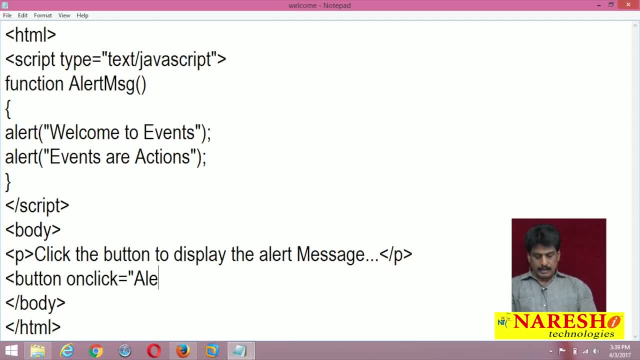 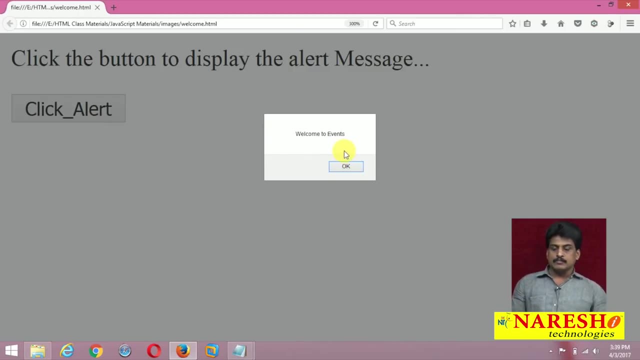 important. I just use slot Chinese, All right. All right, So всем Sesame beğen in-board. Thank you, Bye, Bye. Event. that one alert message: click underscore. alert button: Now refresh. click on that. welcome to events. click. okay. 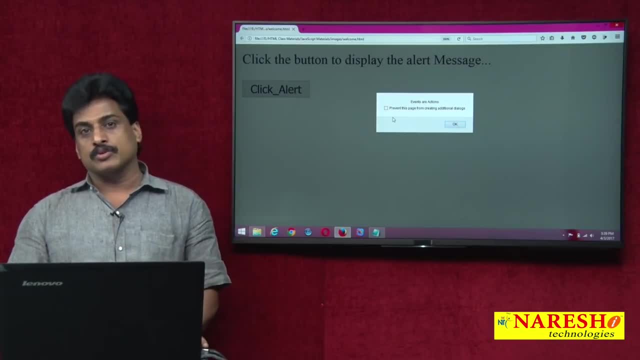 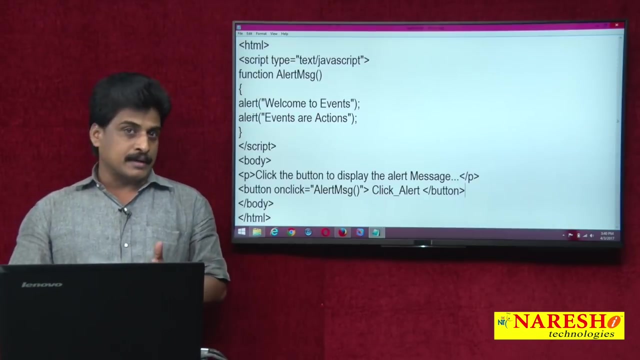 Two alert messages, one single click event, which I have shown to you Not only here, several examples we can do. Click is very most popular event in our JavaScript environment, But basic level example I have shown to you. For example, if you are coming to on click level only, 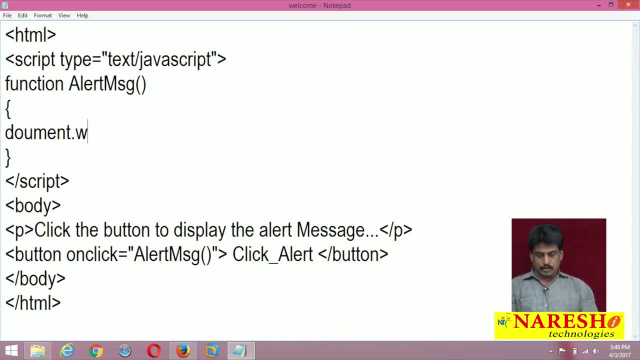 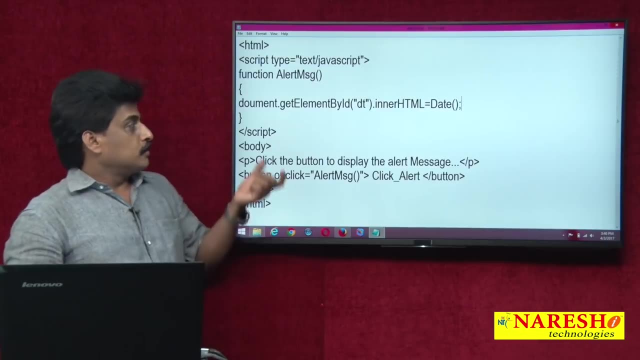 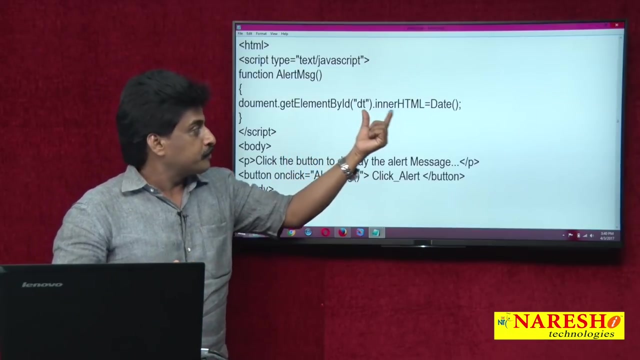 little critical level. we can see Document dot: get element by ID ID I am giving dot. nrhtml is equal to date. Here are several things I need to explain. Document Get element by ID is an object, get element by ID is the method and ID name. nrhtml is the property. date is the function. 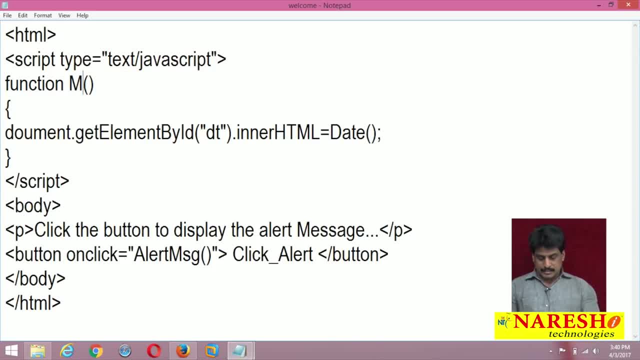 Now I need to change that function name also. I said simply my sysdate. Then come down paragraph: level ID is equal to date. Click the button to display the system date and time. System Date And Time Button on click is equal to what? that one my sys date. okay, 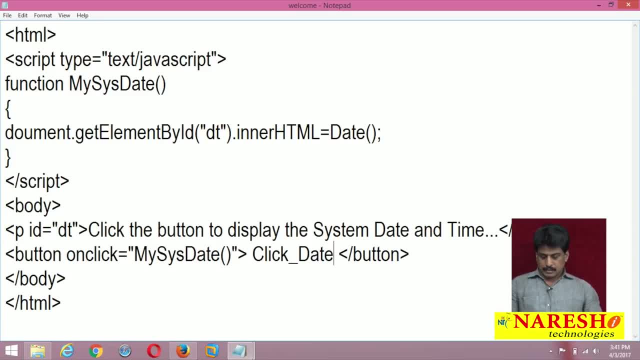 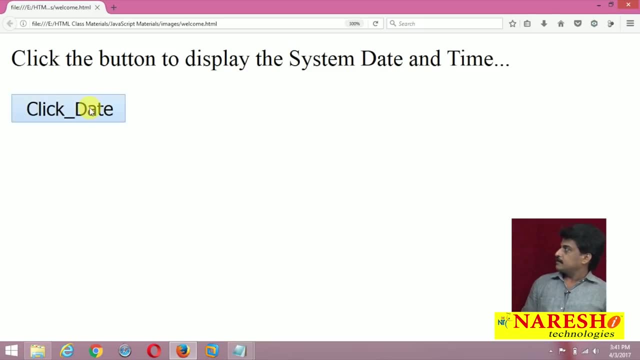 Click underscore date. okay, Now I am going to display that If I click the button it is going to call this function. Function name is my sys date and displaying or not. we can see Write refresh it. Click on that and not displayed. 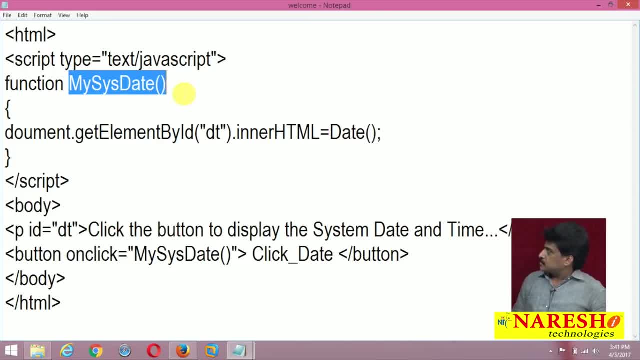 So click the date I said Come down Function. my sys date got correct and ID is equal to date used My sys date you implemented Whenever. click the button to display the system, date and time you are going to call. actually. 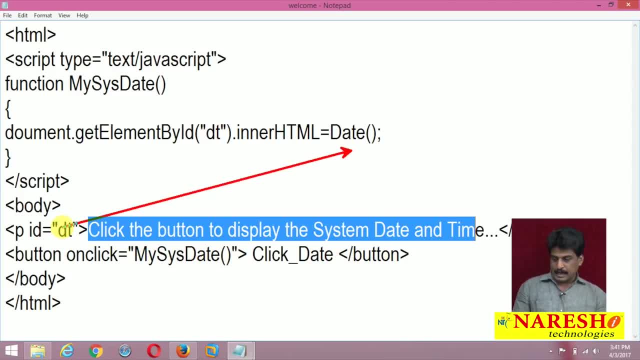 this where? yes, based on ID. Now my sys date is there correctly, observe here. So if you are clicking on that, It should display. But why this innerHTML story? you displayed actually. So document dot level: you can observe before innerHTML spelling mistake. you did already. 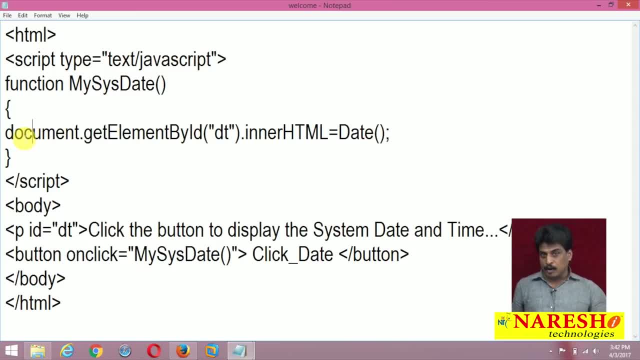 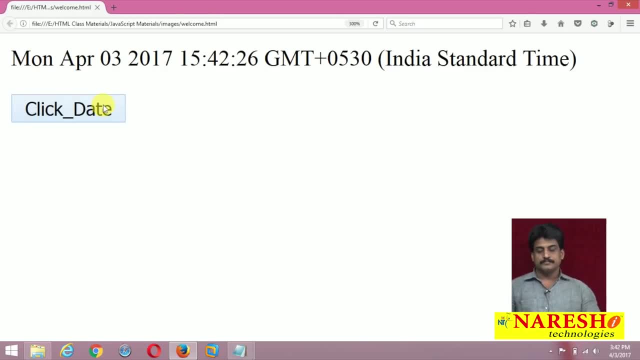 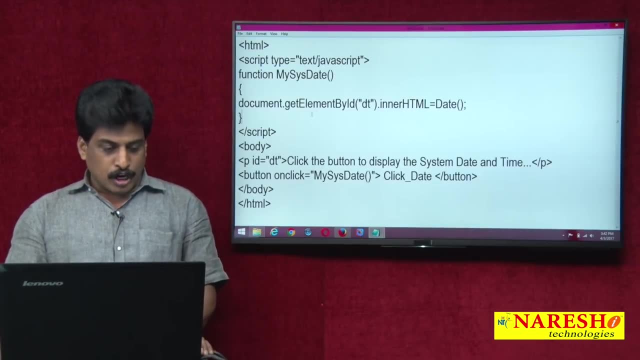 Yes, you need to. What I said, document is an object and which contains getElementById method perfectly displays. now Type mistake, That's all Nothing. is there No logical mistake? Now we can go back. So document dot- getElementById method, innerHTML property. 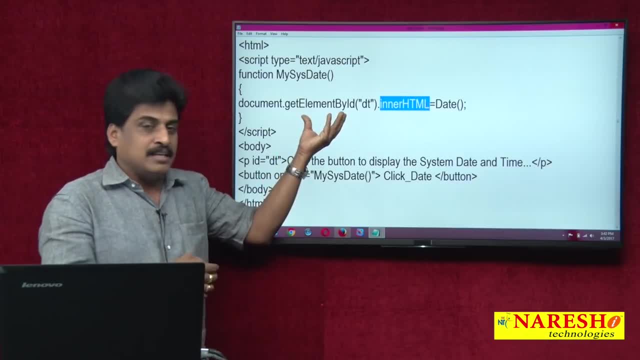 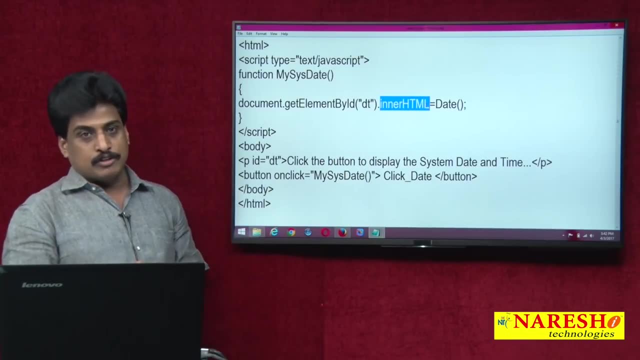 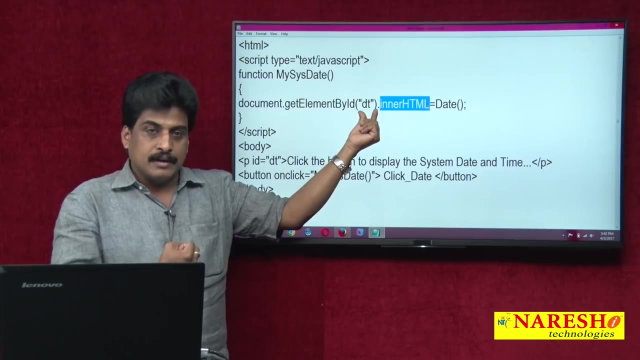 So main you people ready to ask the question: What is this getElementById? you didn't explain What is this innerHTML? we don't have idea, No problem, So methods separately. I will take a video session, But need to understand. from a web page you want to get one element based on ID and that 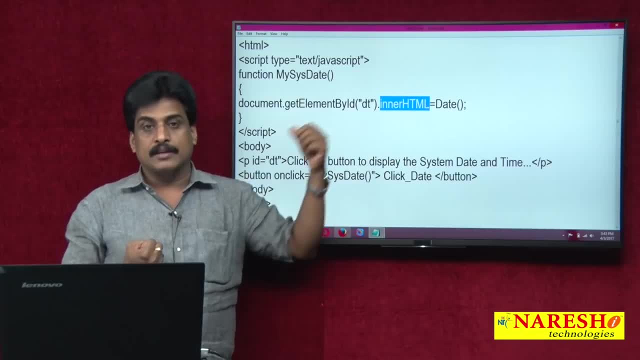 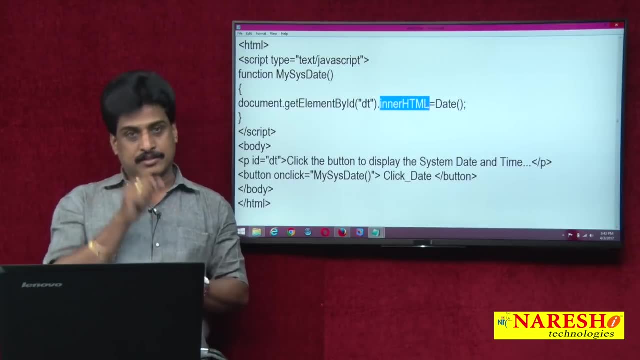 you can get uniquely based on the property Value property InnerHTML. property InnerHTML generally contains for container tags. Value contains for only non-container tags. What are the containers? What are the non-containers? After events, I will show you. 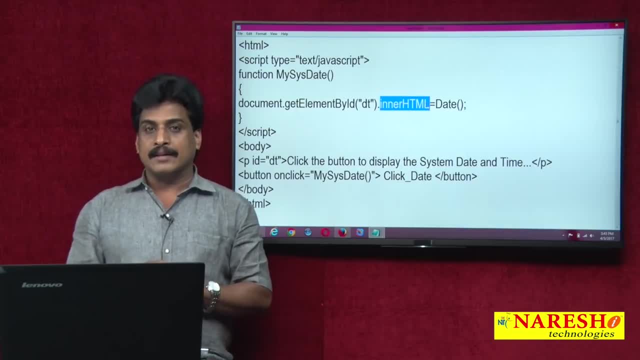 Just in this example. my main motto is: not only alert. we can display other examples also. Come back Now, not only on click. Come down to on double click. Yes, when it is going to fail. Yes, Now it is going to fail. 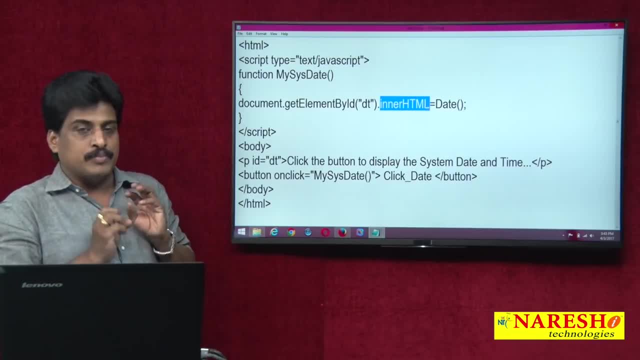 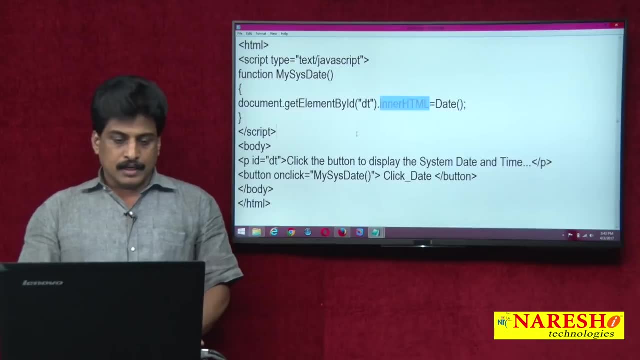 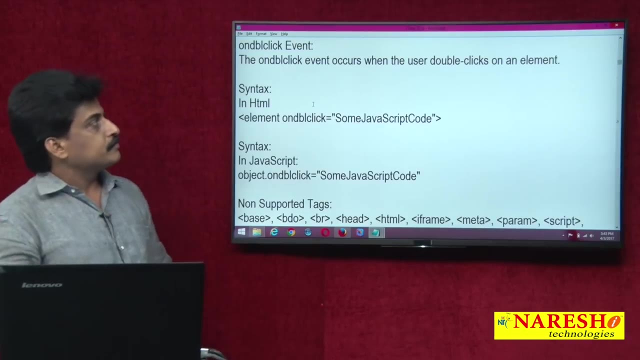 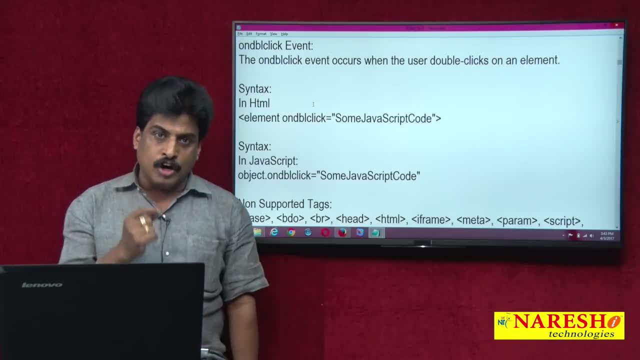 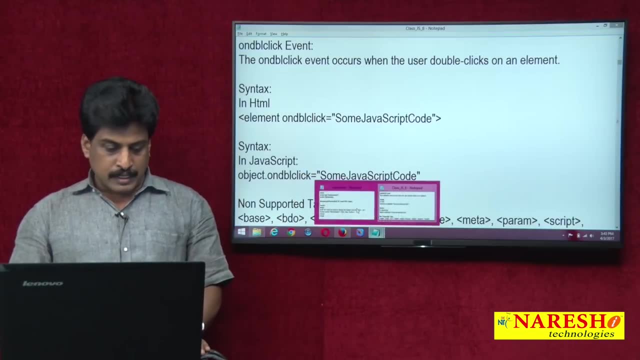 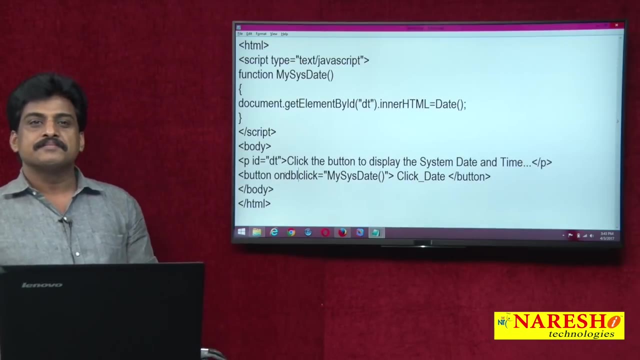 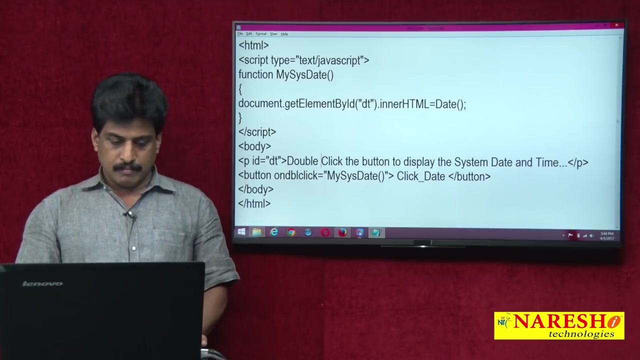 This event occurs when the user double clicks on an element. Simple, Same, almost a syntax, Some JavaScript code, some JavaScript code. Now come down and I am going to display my system on DBL click And I said, on double click, Refresh. 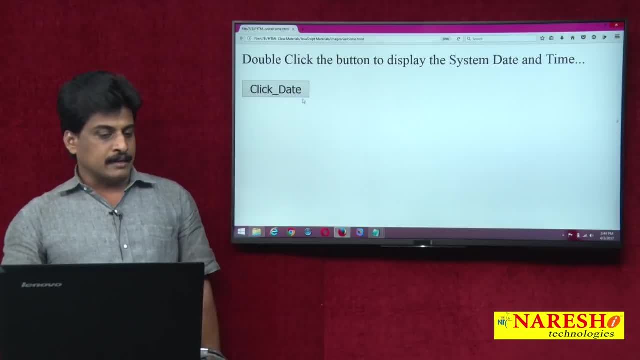 Ok, Ok, Just click on that. Sorry, unable to What event? you implemented here Double click implemented Type. That means I have clicked on the double click, Perfectly displayed. So click click level executing. Double click, double click level executing. 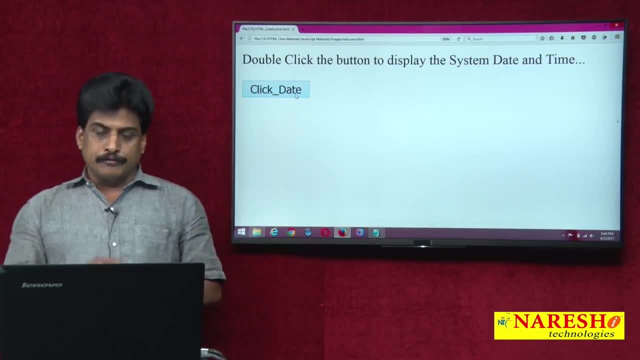 Some kind of requirement I am finding. If you click okay, is there Okay, if you click, automatically convert into cancel some web pages. If you double click on cancel, page will be closed, Like this also events we can develop, But first we will complete the basic events, then we will come back. 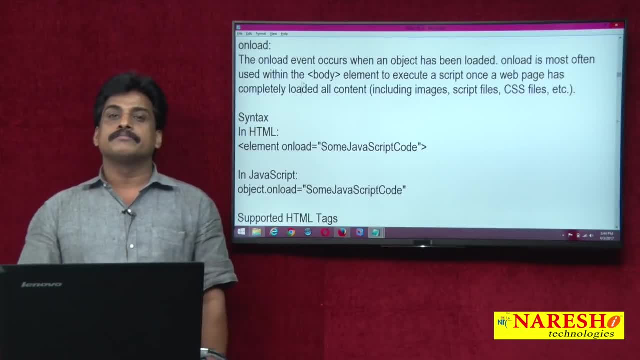 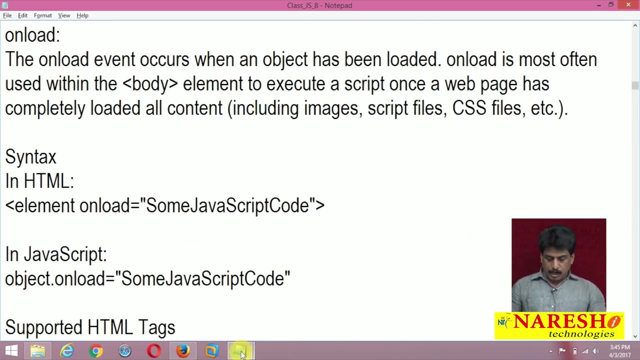 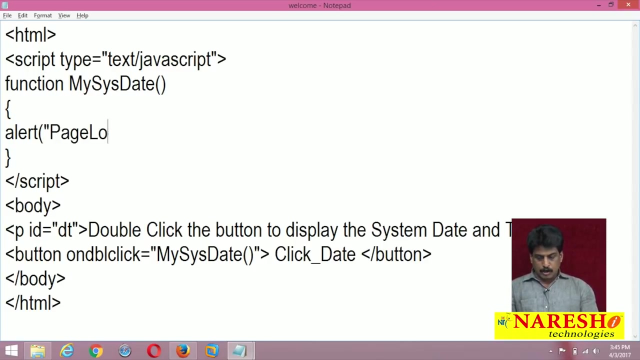 Now I am showing next event On load- Beautiful event. This event occurs when an object has been loaded On. load is the most often used way Within the body section. Commonly we are using Including images level also. we can use Script level also. we can use And syntax element level as well as object level. Right on load event. I am performing Simply first one alert message. I will show you Alert page loaded successfully Right. close that. And page load related names. I am providing Page load. 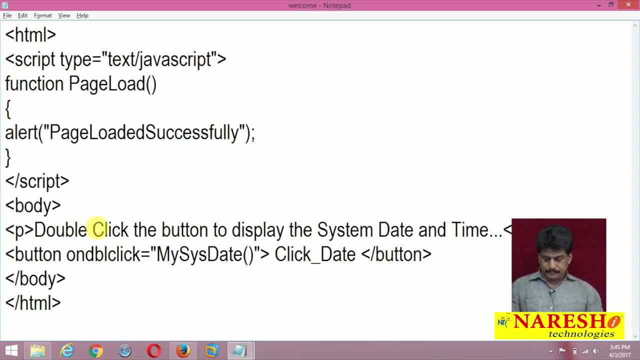 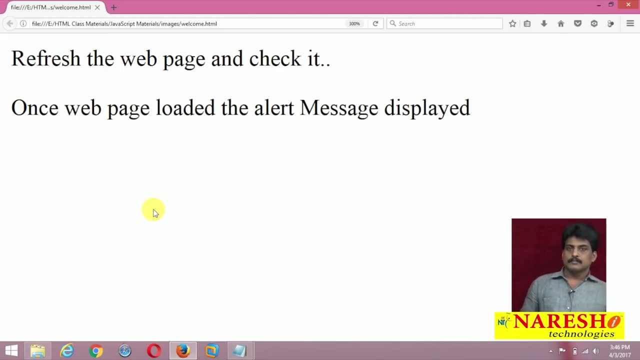 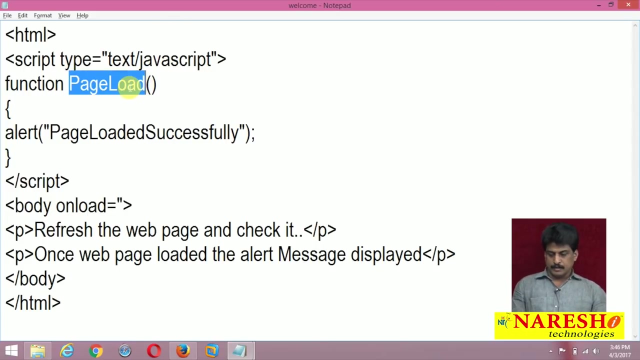 Now. just you can try to refresh that. Refresh the web page and check it. Once web page loaded, the alert message displays Come on refresh. Not displayed Where you wrote on load. Yes, body level On load equal to What is that one Page load? You need to call that. Yes, Come on refresh now. 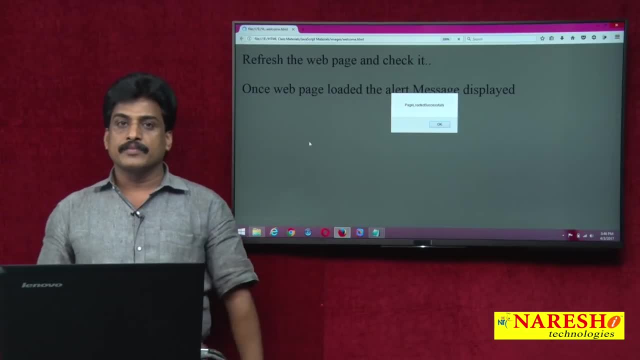 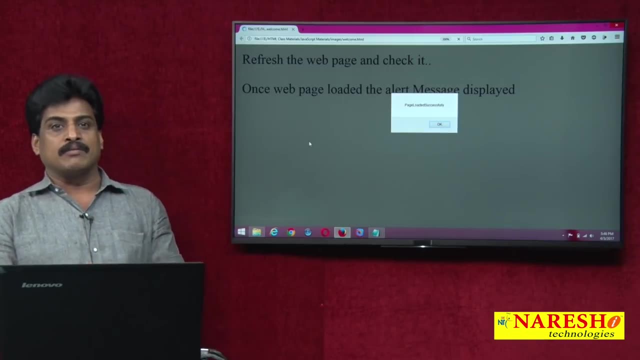 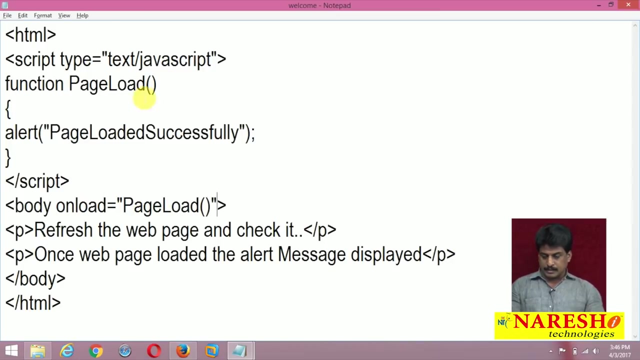 Perfectly. Page loaded successfully. Actually this page load when the server side response is there. effectively we can, But I am not teaching to you any server level programming, Just client level JavaScript At the browser level. I am trying to show you. But same example: little effectively we can do. For example, one image I will take, Image loaded successfully. So one image I am taking, Image loaded And image just to alert.